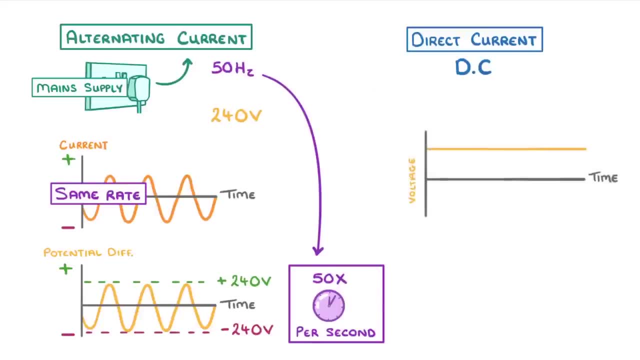 Direct current, on the other hand, is produced by a direct potential difference, which is either positive or negative the entire time, So the charge is always flowing in the same direction. We find direct current in things like cells and batteries, like those in your phone or 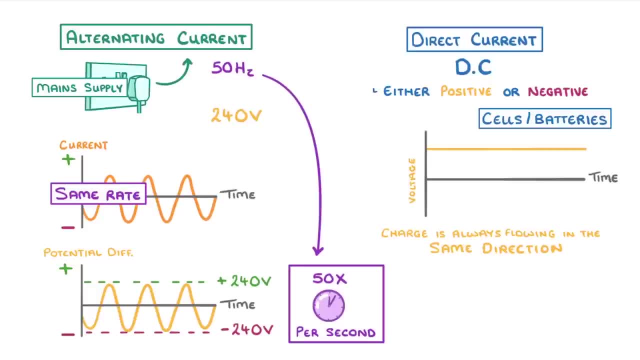 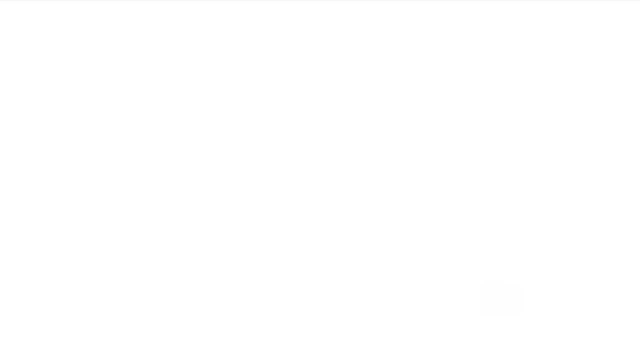 a calculator. The last thing we need to cover is that, in order to get these potential difference vs time graphs, we use devices called oscilloscopes, which display the graphs on a monitor. Anyway, that's everything for today, so hope you found the video helpful. If you did, then. do share it with your friends and we'll see you next time. 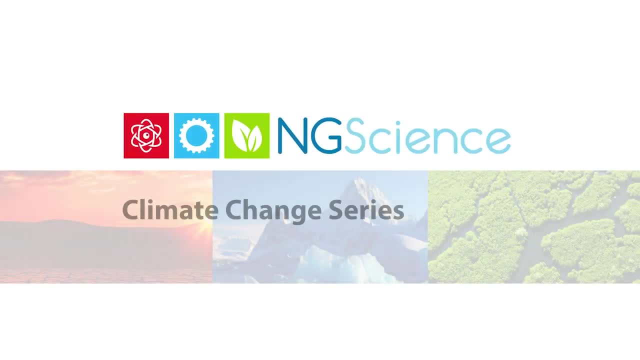 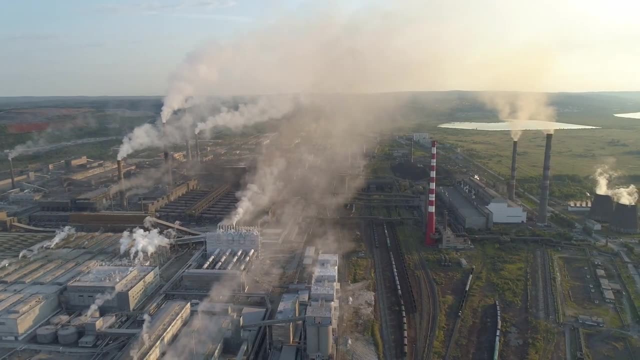 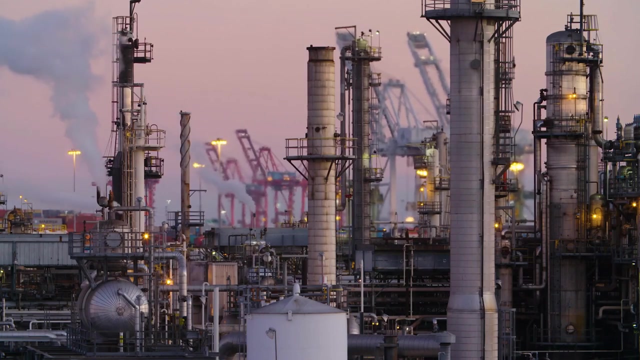 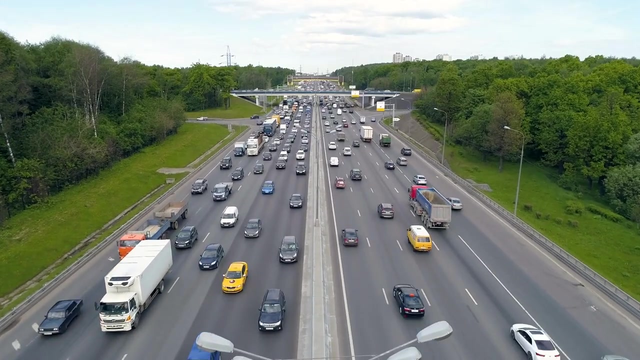 For generations, humanity has relied heavily on fossil fuels like coal, oil and natural gas to power our lives. These sources have given us the energy to light up our cities, drive our vehicles and run our factories. But there's a dark side to this dependency. 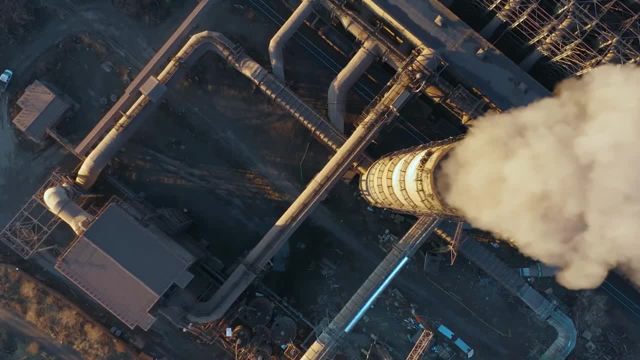 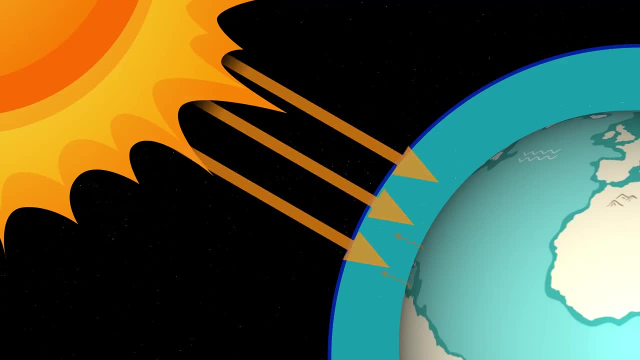 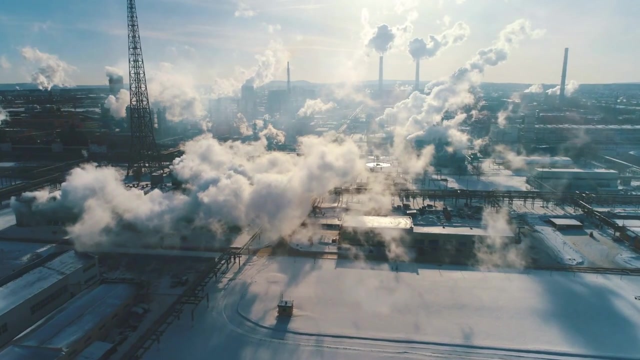 Burning fossil fuels releases carbon dioxide and other greenhouse gases into the atmosphere. Over time, these gases have accumulated, creating a thickening blanket around Earth that traps heat. This phenomenon, known as the greenhouse effect, is the primary driver of global warming and the resulting climate change we're experiencing today. 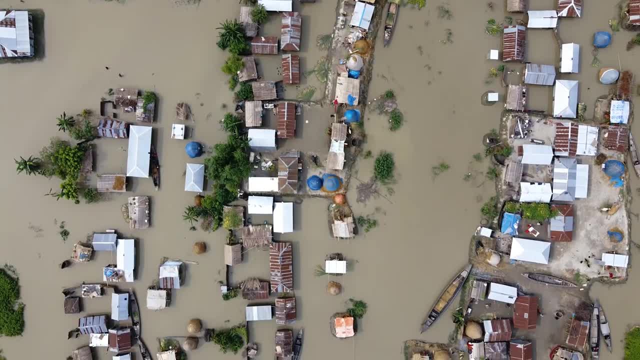 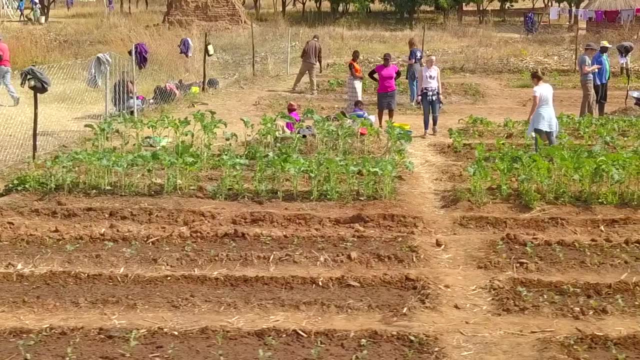 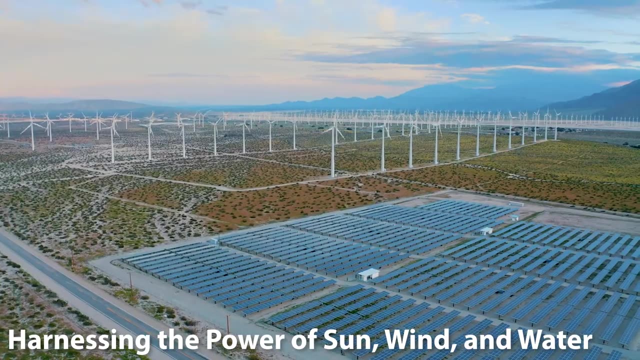 This change manifests as extreme weather patterns, rising sea levels and shifts in global temperatures, all of which have serious implications for our planet and its inhabitants. So what's the solution? Enter renewable energy, Harnessing the power of sun, wind and water. 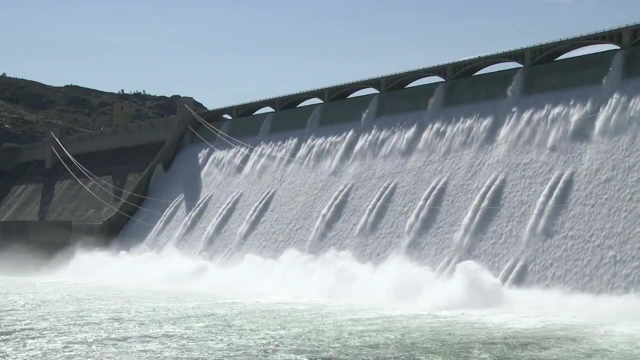 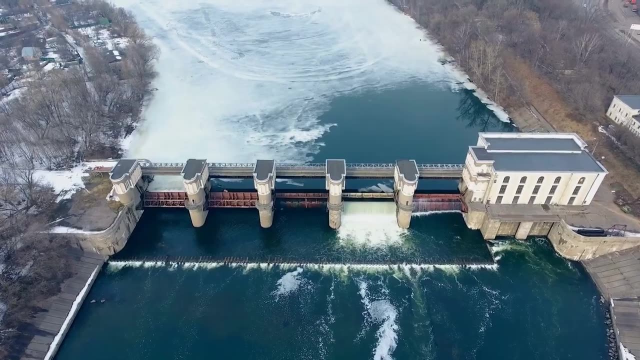 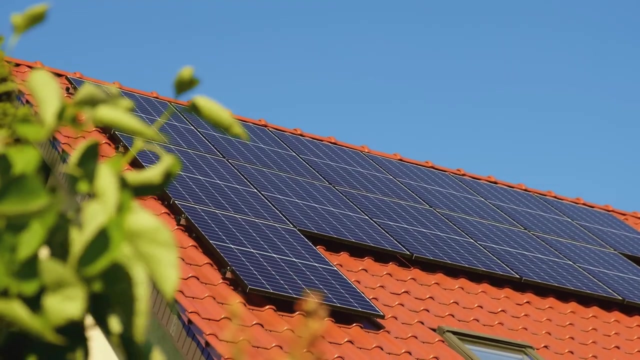 Renewable energy sources like solar, wind and hydroelectric power offer a sustainable alternative to fossil fuels. These energy sources are called renewable because they won't run out in our lifetimes, unlike fossil fuels, which are finite. Solar panels capture the sun's energy.